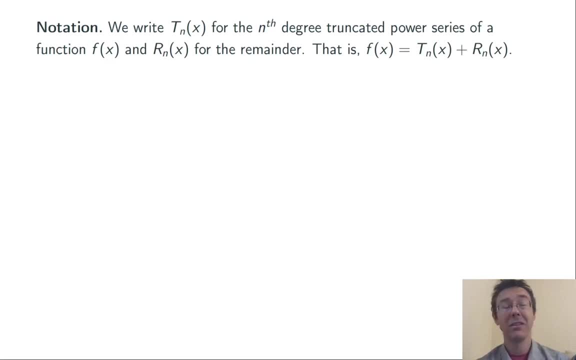 of the series. So then, the function f is the sum of capital T and capital R. Remember that capital T is just a polynomial, while capital R is going to be an infinite series. just missing the first few terms, We have two real, two basic tools for estimating error. 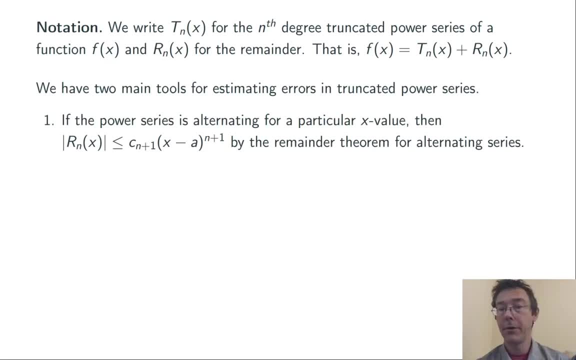 First of all, the remainder theorem for alternating series. Obviously, this only works if the power series that you have is alternating for a particular x value And it basically just says: look at the next term of the series If the series is going to be alternating for. 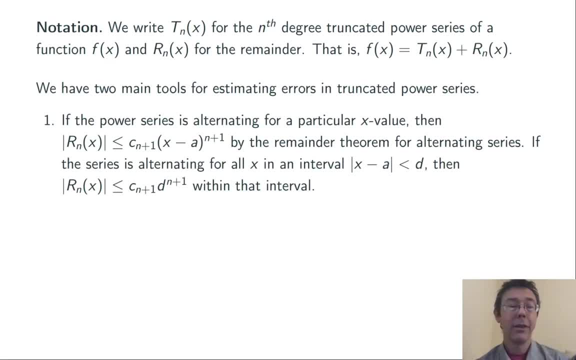 all x values in an interval around the center. then we can just use sort of the worst case scenario- Let x minus a equal d and plug into that previous approximation Again, that only works if the series is going to be alternating for every value of x within. 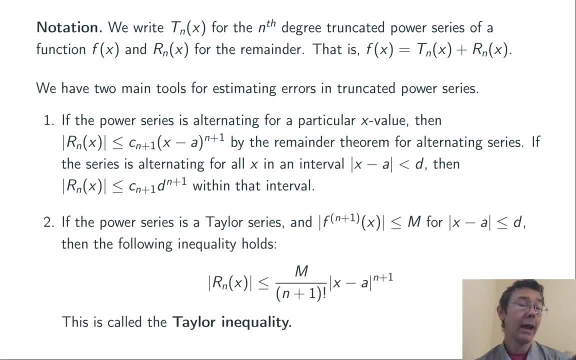 that interval. The second tool we have is the Taylor inequality. So this is particular to Taylor series, not just the power series in general. Roughly speaking, it also says to look at the next term in the power series after the ones, after where you've truncated. 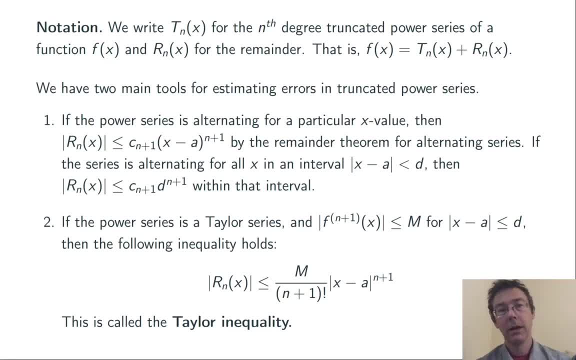 it. So the first term of capital R sub n. Here though it's a bit more subtle than just using a particular x value Or just using an n point on that interval. So the m over n plus 1 factorial is going. 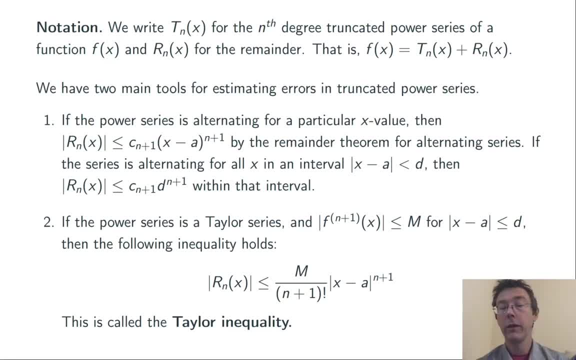 to look a lot like the Taylor coefficient, which is the n plus first derivative evaluated at the center. Here, however, when we're doing the Taylor inequality, we can't just evaluate it at the center. We have to take the value that makes that as large as possible. on that, 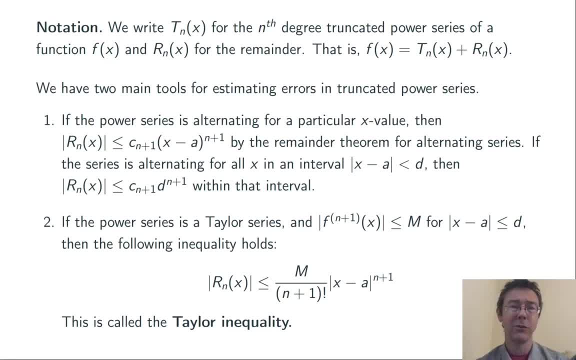 interval. We'll call that value capital M. It kind of stands for maximum. By the way, this inequality will still hold if we take a value larger than that maximum. but in general we'll try and find an actual maximum value on that interval. 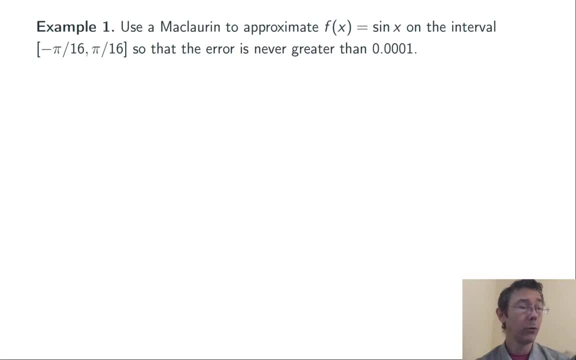 This all gets clearer when we start doing examples. So let's do two. Number one: use the McLaurin series to approximate f of x, equals sine x, on the interval negative pi over 16, comma, pi over 16, so that the error is never greater than 0.0001.. So first of 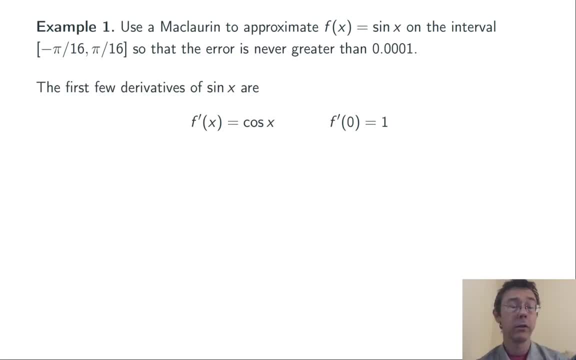 all. we need the McLaurin series, In other words the power series centered at 0.. We need some derivatives. So the derivatives go cosine x, negative sine x, negative cosine x sine x, and then it starts repeating And 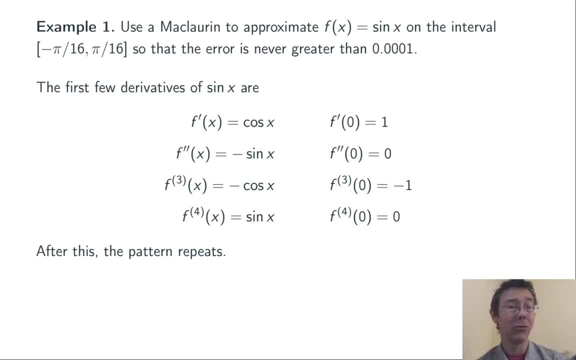 when we plug in 0 to those, we get 1,, 0, negative 1, and 0 for our first four derivatives. So the first few terms of the McLaurin series for sine x are going to be x minus x cubed. 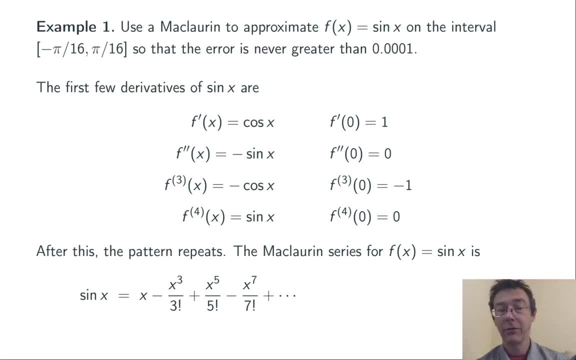 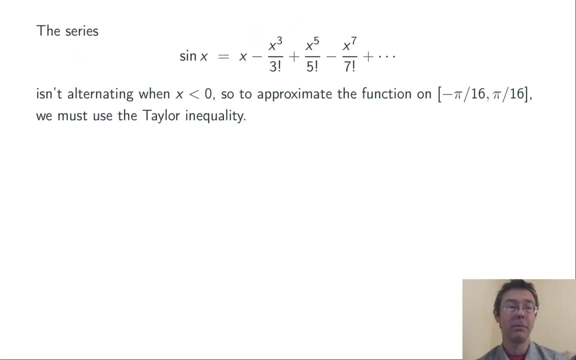 over 3 factorial plus x to the 5th over 5 factorial minus x to the 7th over 7 factorial. Here's the more general formula for sine x, for the McLaurin series for sine x, although we won't particularly need that for this problem. Okay, so this may look like an alternating. 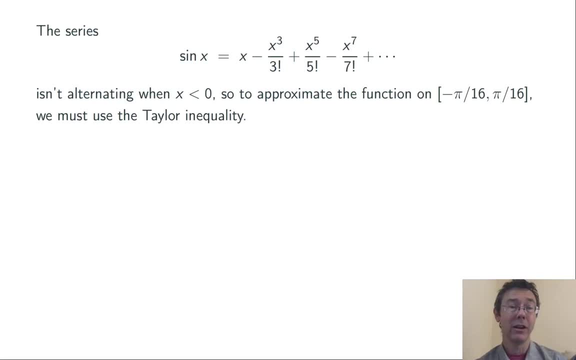 series, but when x is negative it's not alternating. So we're going to have to use the Taylor inequality. Here it is again. We need two things. First of all, we have to deal with the x minus a to the n plus 1, and also substitute out the n plus 1 factorial, and then we need to 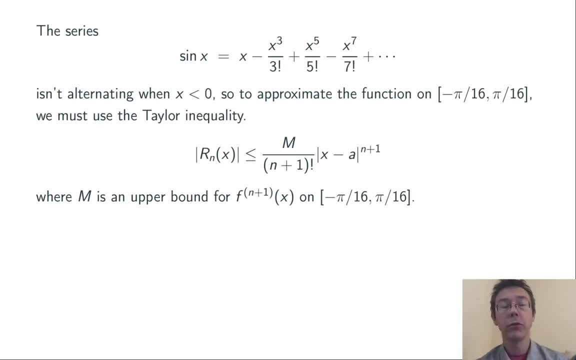 find an upper bound m for the n plus first derivative on that interval. So first of all, just plugging in for the other things, n is 3 here, so that's where the 4's are coming from, and a is 0. So the largest that x minus a is is 1, and the last largest is n. So there's. 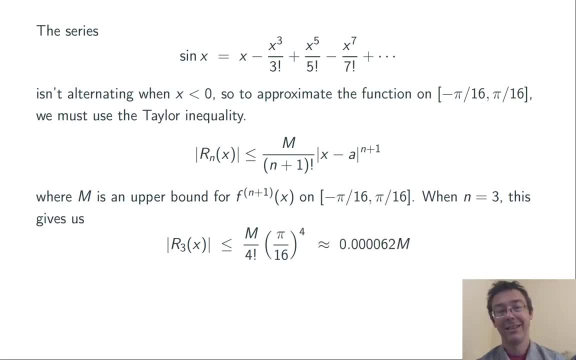 this: a can be on this interval is pi over 16.. Roughly, I'm getting point zero, zero, zero, zero, six, two times m. Now, m is going to be fairly easy to find here, because the fourth derivative is sine of x, and sine of x is never greater than one. Now, if I were to, if I needed to be a bit more, 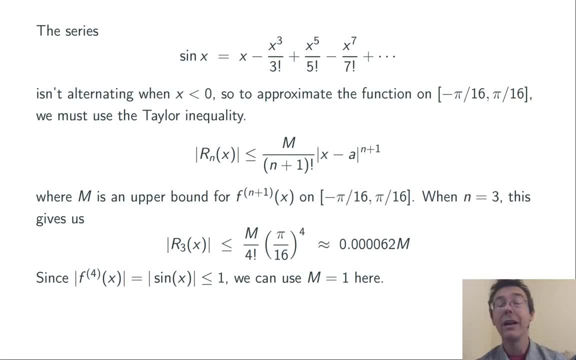 accurate. I could restrict my attention just to this interval and even get a smaller value for the maximum that sine can be. Here I just plug in one and then even just using the first two non-zero terms of that Maclaurin series, I get that the series approximation is going to be. 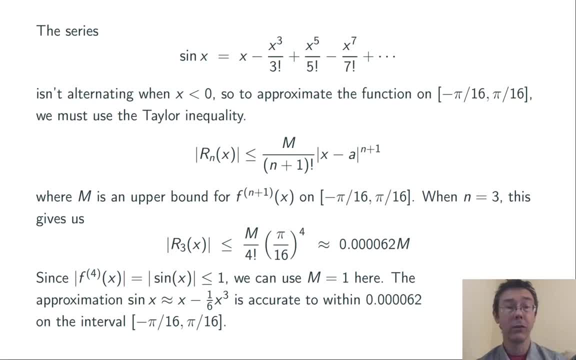 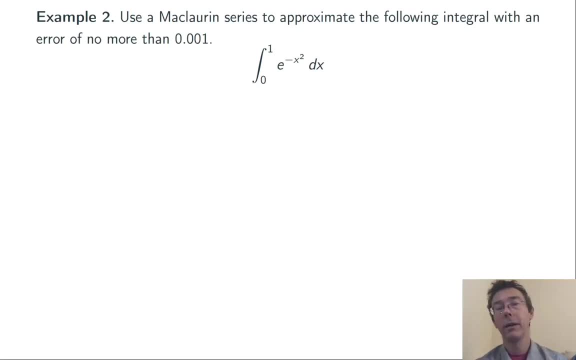 accurate to within point zero zero zero zero six two on this interval. Example two: Use the Maclaurin series to approximate this integral with an error of no more than point zero zero one. Okay, so the function e to the negative x squared does not have an elementary antiderivative. We can't just write: 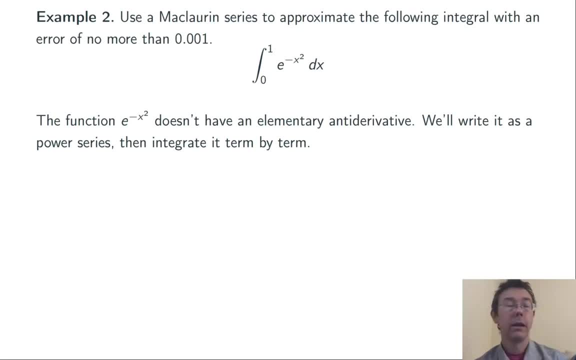 down a function that has that derivative. So we are not going to be able to directly apply this fundamental theorem of calculus. Instead, what we're going to want to do is to write e to the negative x squared as a power series, integrate it term by term and then plug in those end points. 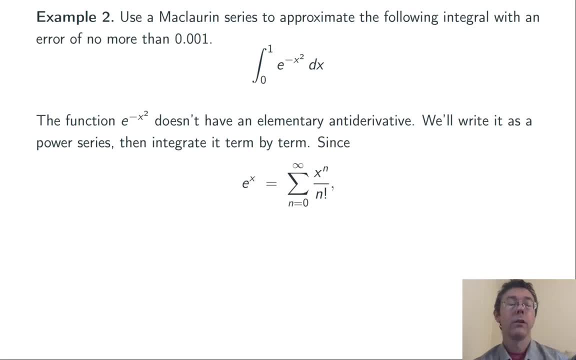 and then, of course, approximate the error. So instead of just doing derivatives directly and then just applying the fundamental theorem of calculus, we're going to want to write e to the source feet and calculate in the Maclaurin series directly. I'm going to 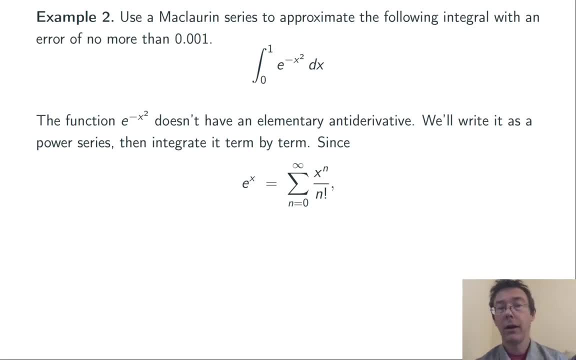 start with a power series for e to the x, Which is pretty standard, the sum of x to the n over n, factorial. And then I'm going to take out the x and replace it with negative x squared, Simplifying that a tiny bit, I get: the sum from n equals zero to infinity. negative one to the n. 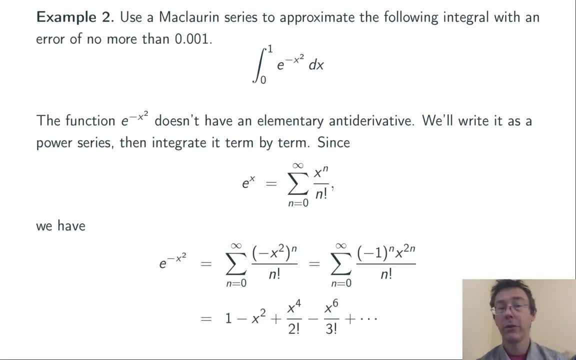 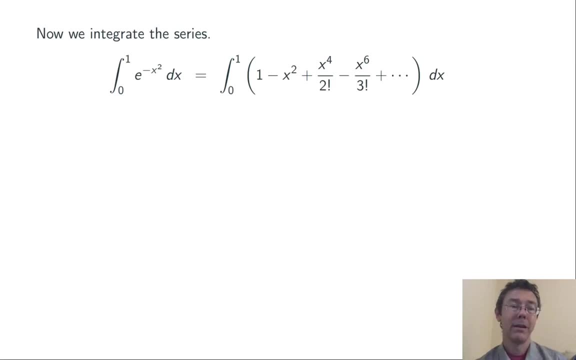 x to the two, n over n, factorial. Here's the first few terms: one minus x squared plus x to the four, minus x squared plus x to the fourth over two, factorial, and so on. So let's take out e to the negative x squared and replace it with the power series. it's: 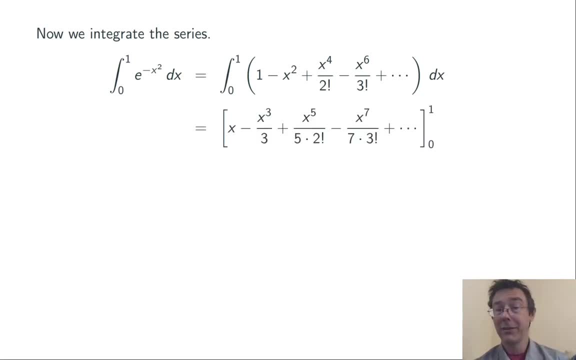 equal to, and then integrate term by term and plug in the endpoints. So the integral from zero to one, e to the negative x squared, is going to have this numerical value and just by adding more and more terms we can get better and better approximations. 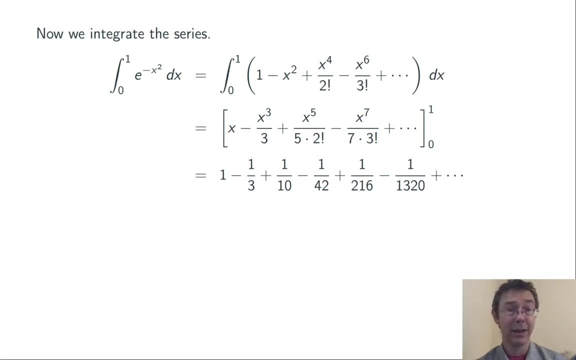 In theory, if we could do that whole sum, we'd get the exact value of that definite integral. Okay, so this is an alternating series, and so we can approximate the error e sub n. rather we can bound it above using the absolute value of the n plus first term. 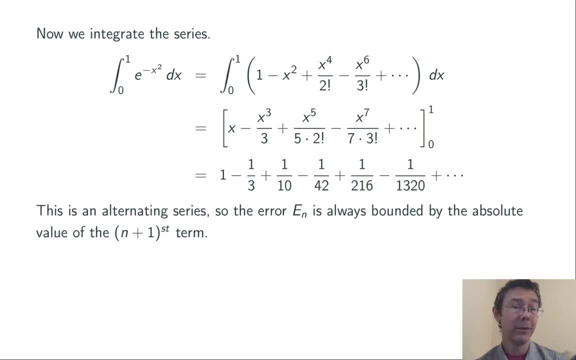 So if I add up n terms, I take the absolute value of the following term, and I know the error is not going to be bigger than that absolute value. So, for example, The sixth term in this series in absolute value is one over one thousand three hundred.